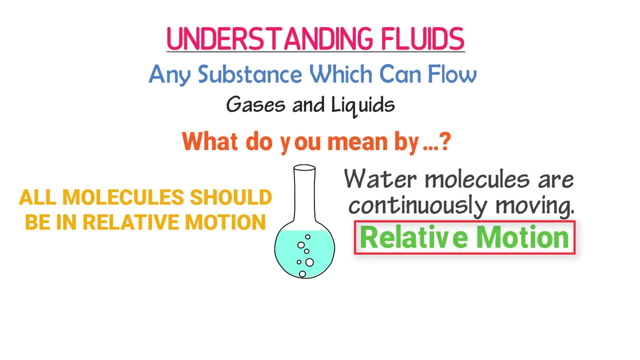 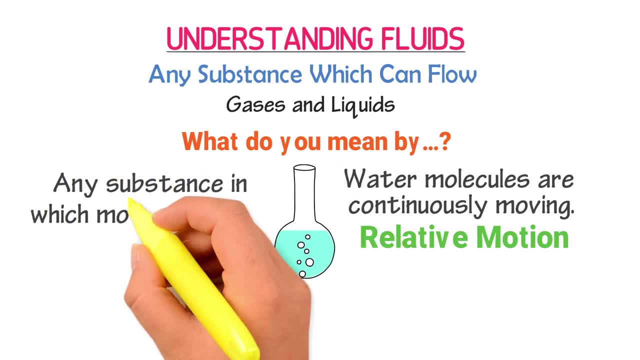 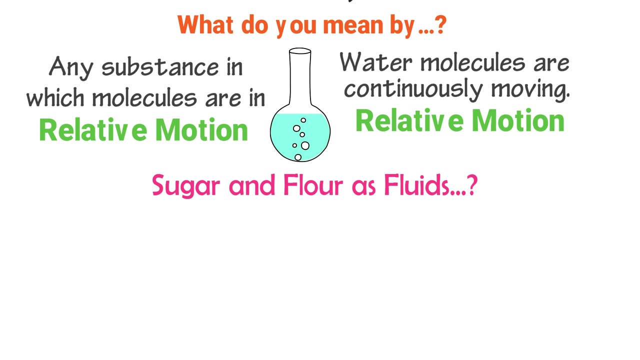 The third definition of fluids is: any substance in which molecules are in relative motion or in relative flow is known as fluids. Here let me ask you a question: Can we call sugar and flour as fluids? Because if you tilt a glass of sugar or a glass of flour, 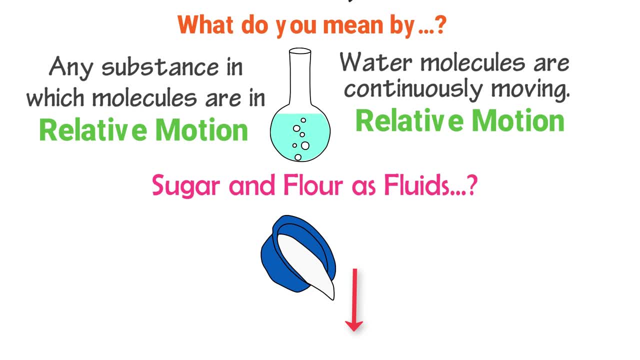 they both flow in downward direction. Can you guess the answer? Well, the answer is no. The molecules or particles of sugar and flour do not change their respective position with the passage of time. Hence, they are not fluids, They are solids. They 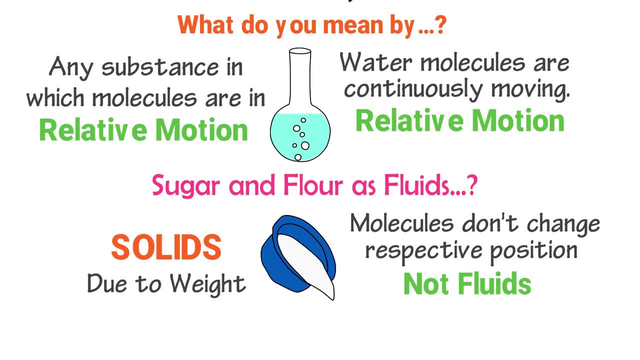 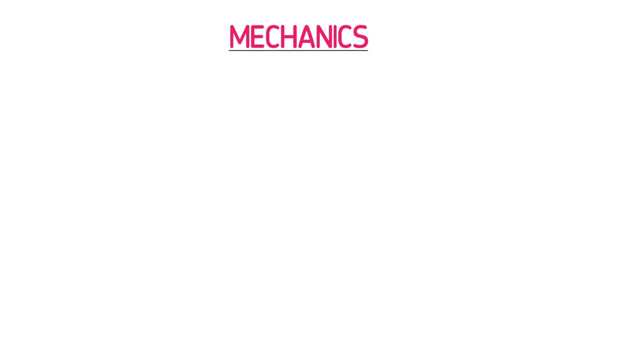 fall off from any object due to their respective weight. Now let me also clear your concept of mechanics. Mechanics is the branch of science in which we study about force and its effects. By effects I mean magnitude of force, direction of force, etc. For example, consider a stationary football. When you kick it, you exert force. 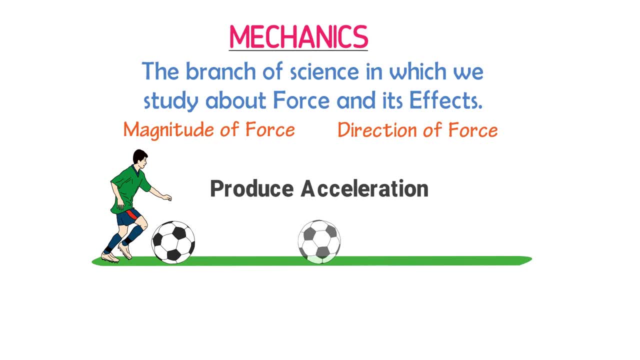 on it. Force produces acceleration in it. Thus, remember that in mechanics, we study about force and its effects. Now let me also clear your concept of mechanics. Mechanics is the branch of science in which we study about fluid mechanics. Now, what is fluid mechanics? The branch of science? 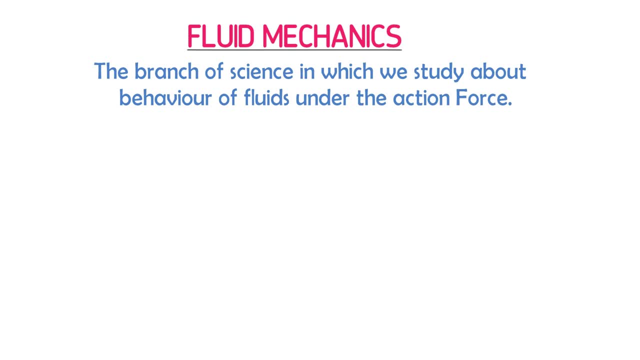 in which we study about the behavior of fluids under the action of forces, is known as fluid mechanics. Fluid mechanics is further divided into three parts: Fluid statics, fluid kinematics and fluid dynamics. Now, what is fluid statics? Well, the word statics means fluid dynamics.